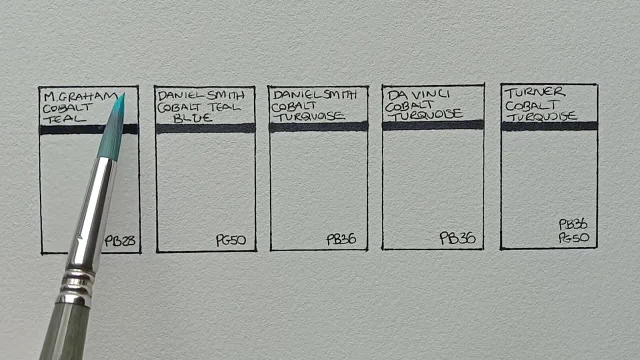 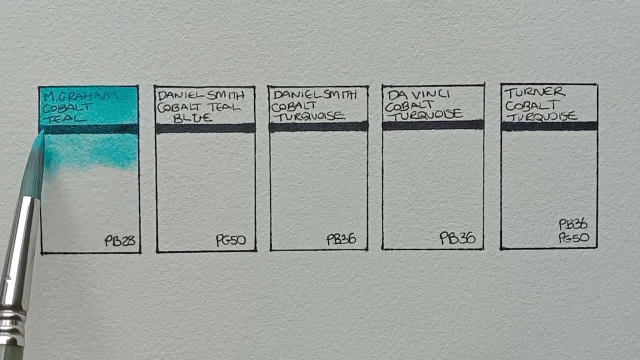 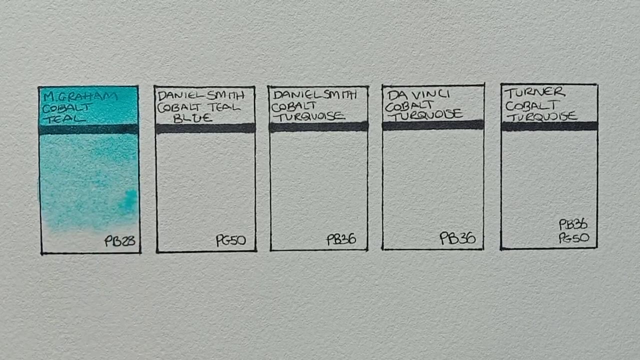 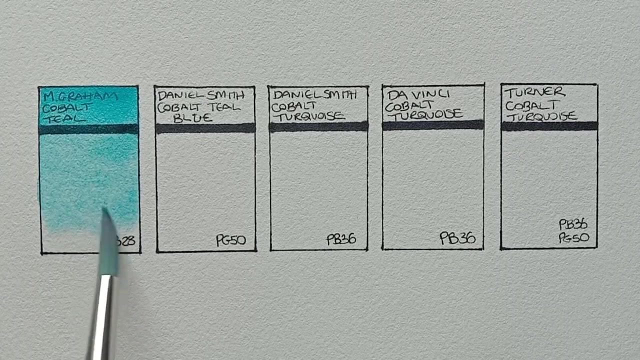 Okay, so first up we have M Graham cobalt teal, and this is made from PB28.. Yeah, I really do like this colour. I don't have all that much experience with M Graham watercolours but, yeah, I think that's going to change real soon. 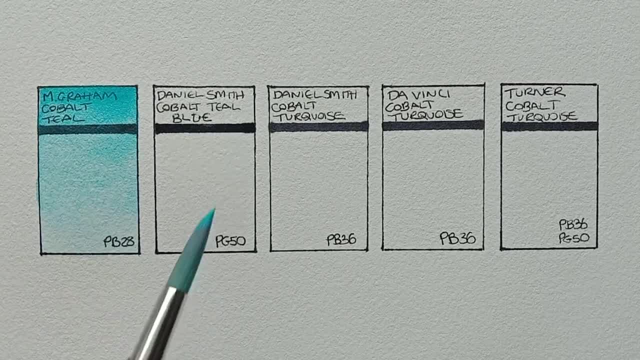 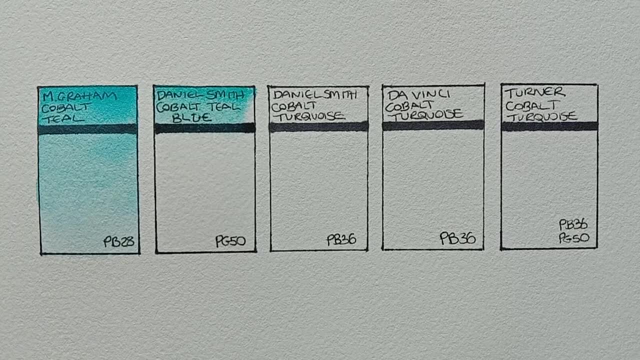 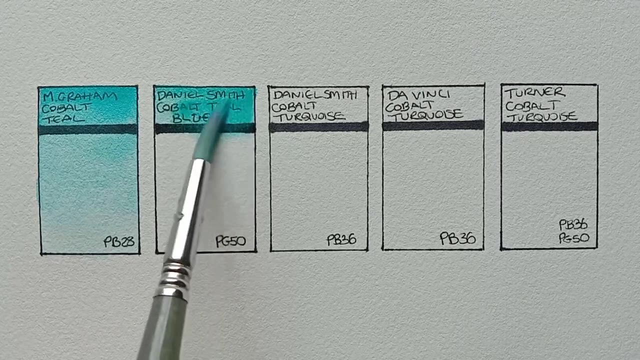 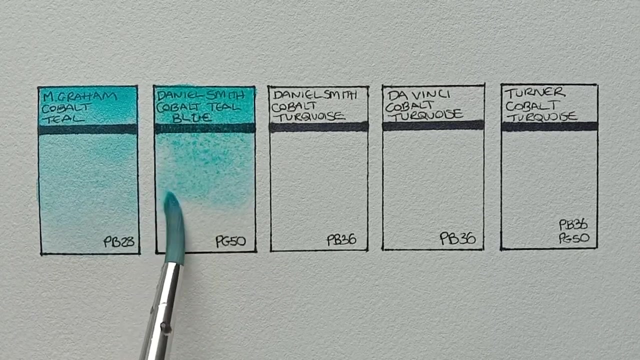 And next we have the Daniel Smith cobalt teal- blue, and this one's made from PG50.. So this is the cobalt teal I hear most people raving about. I see a few landscape artists that I like incorporating it into their work. 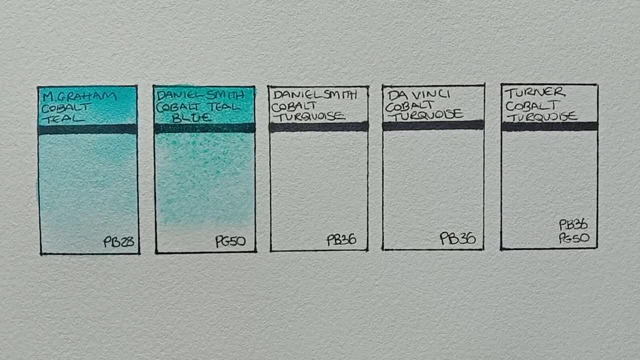 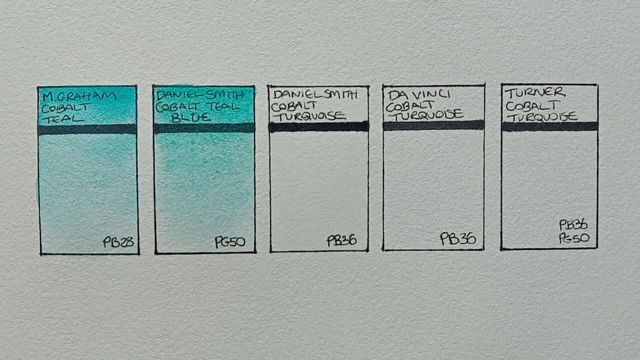 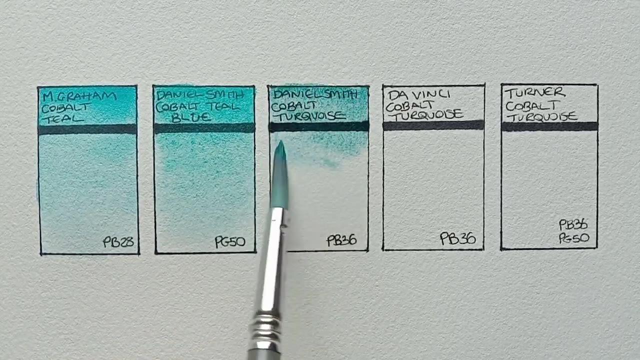 Yeah, it is really nice. It's definitely greener than the M Graham and I think it has more granulation as well. And now we're moving on to the cobalt turquoise paints, And first up is Daniel Smith cobalt turquoise, and it's made from PB36.. 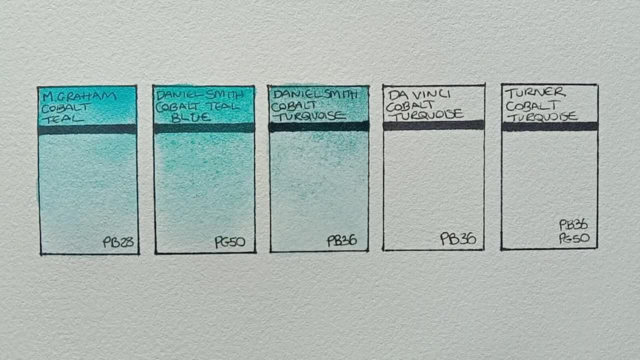 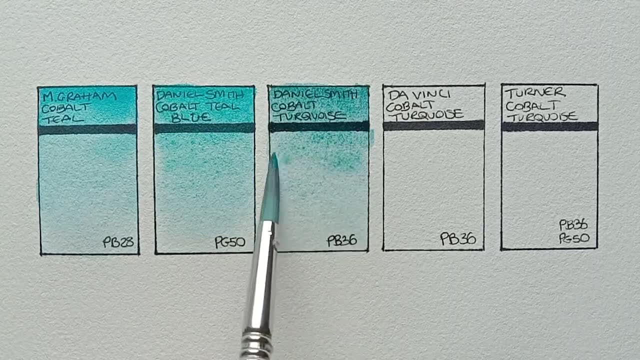 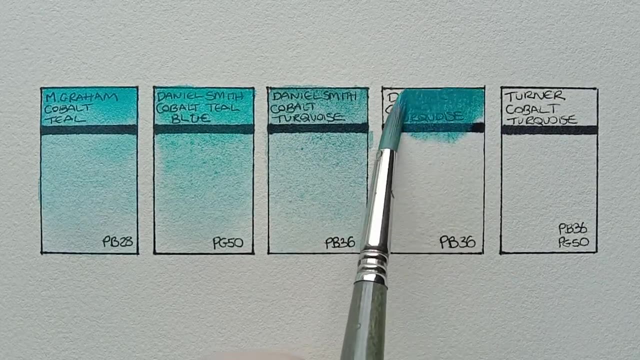 Okay, so I'm seeing the turquoise is definitely greener than the teal. Yeah, It's really nice. I think I might actually prefer this to the teal. maybe Next is Da Vinci cobalt turquoise, and it's also made from PB36.. 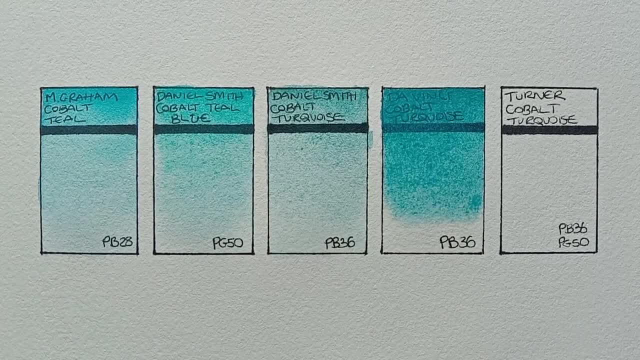 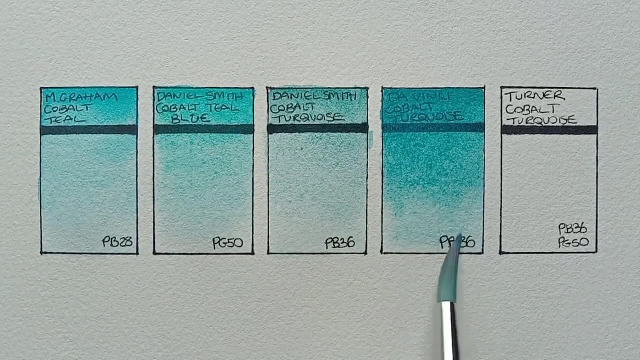 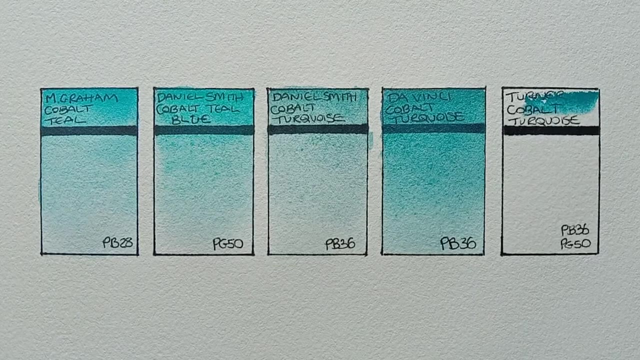 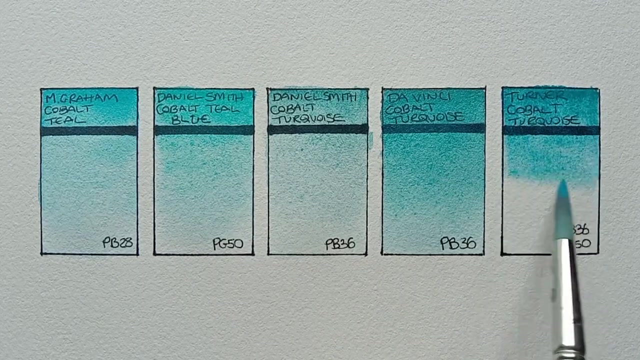 Wow, it's very different from the Daniel Smith before it. Yeah, I think it's still nice, but yeah, I prefer the Daniel Smith, I think. And the final paint here is cobalt turquoise from Turner. Now, this is a two pigment mix of PB36 and PG50.. 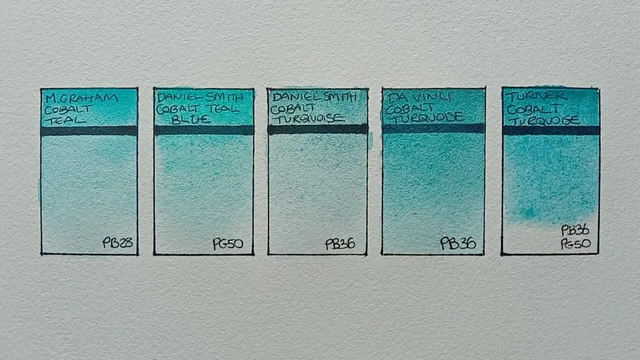 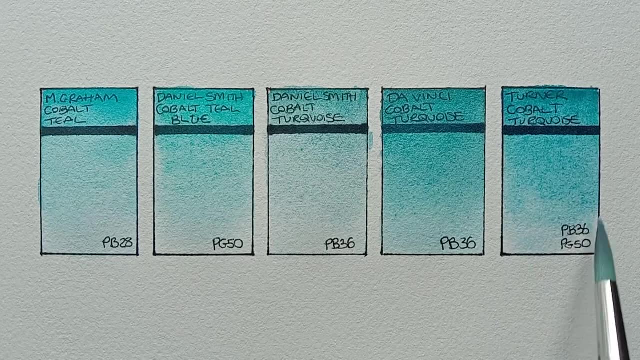 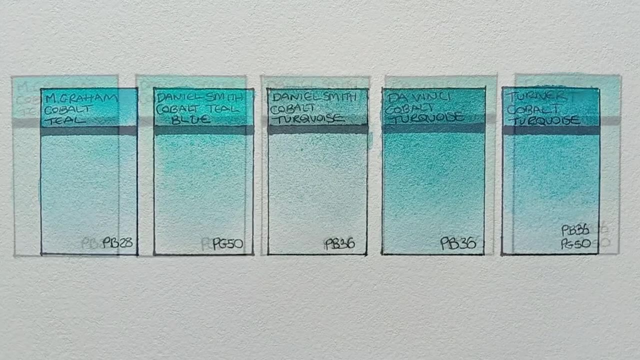 I can see right away that it's bluer than the previous two. Not quite as blue as the M Graham cobalt teal, but yeah, it's not far off. Yeah, I quite like it actually. Okay, that's all of them painted out and here they are in daylight when completely dry.